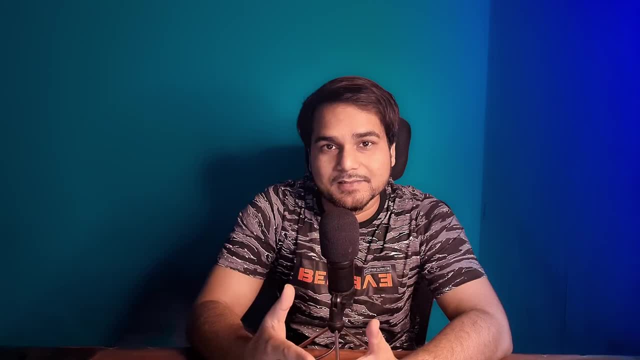 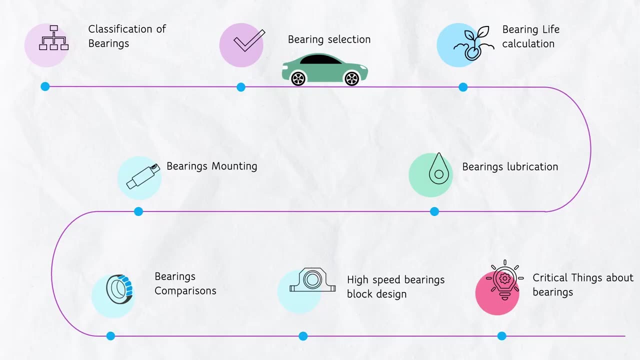 thing that matters. The selection of bearings is not only about selecting the right type of bearing. Bearing selection is also about the selected bearings should meet their expected service life. So we will master the bearing service life calculation. Also, we have to learn the selection. 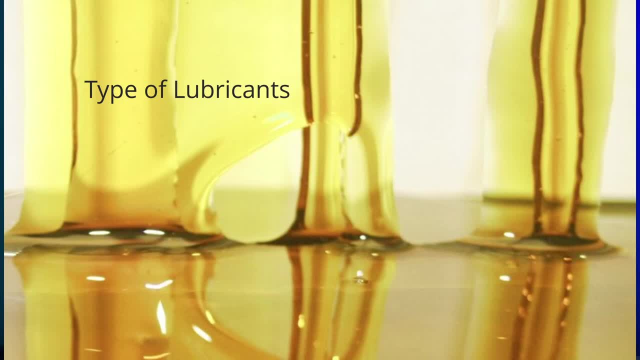 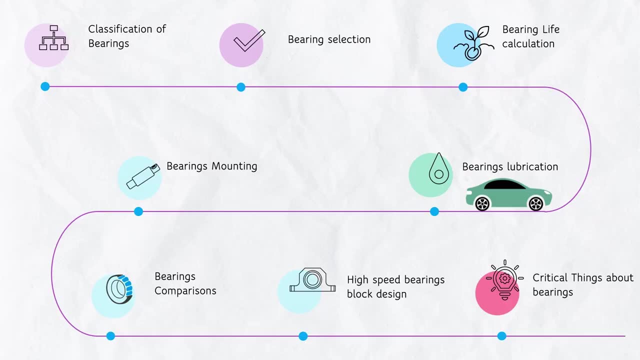 of bearing lubrication, lubrication type and calculation of right amount of lubrication for a bearing. And as per the designer point of view, we have to also master the bearing. mounting That, how to determine the right lubrication for a bearing And as per the designer point of view, 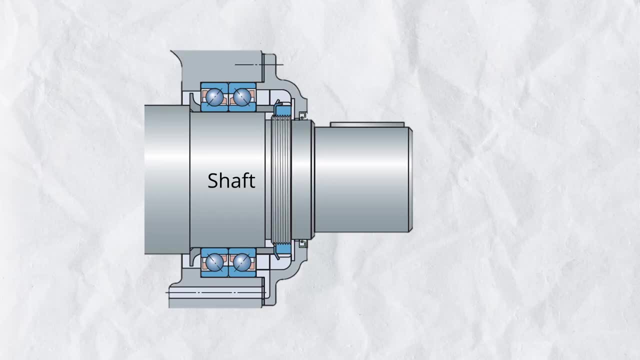 we have to also master the bearing mounting That- how to determine the right lubrication for a bearing. And, as per the designer point of view, we have to also master the bearing mounting That- how to determine the right amount of tolerance over bearing shaft and bearing hosing for different bearings. And I am 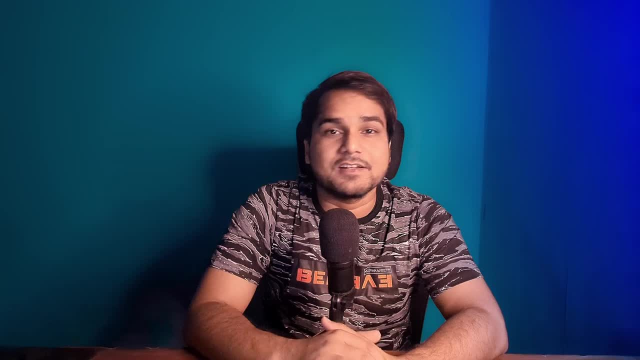 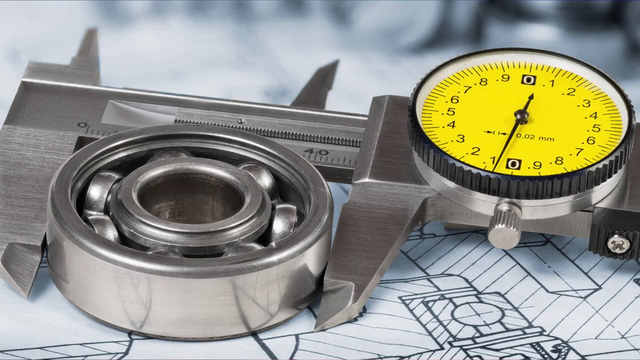 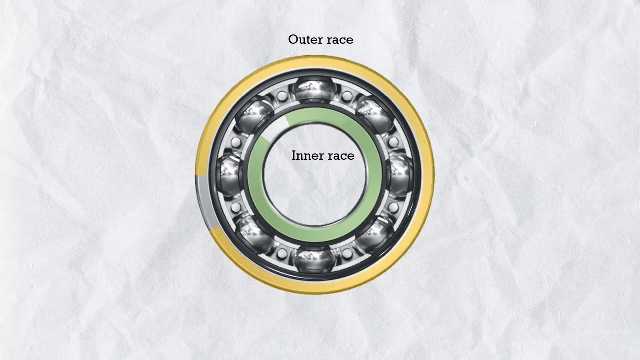 telling you there is no thumb rule. There are many factors that decides the tolerance over bearing seats, Like bearing precision grade means in which tolerance bearing manufacture itself, Also in relative motion, that which part of bearing is moving and which part of bearing is stationary. 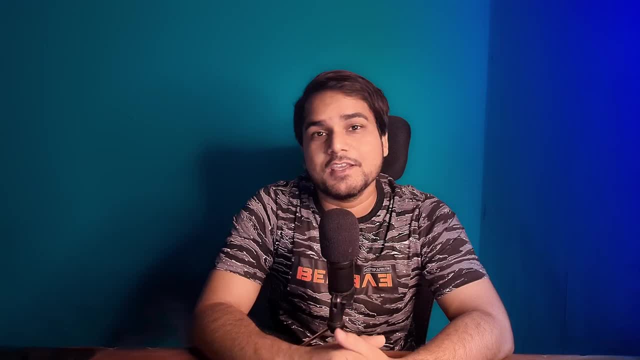 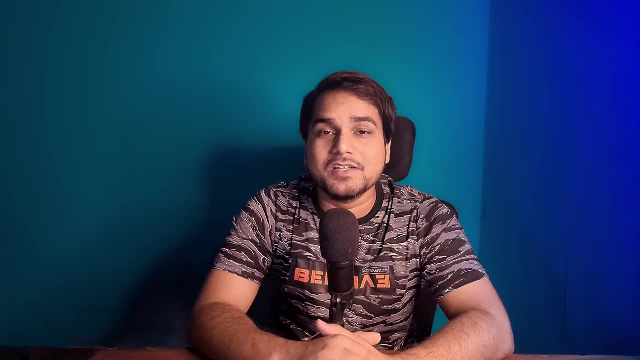 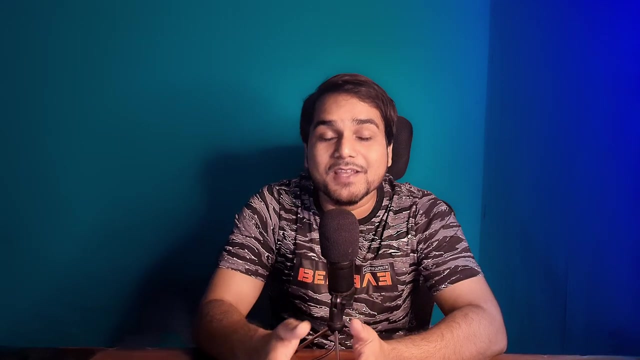 And selection of right fit of a bearing is very important because the bearing fits tolerance directly impacts the bearing life. so again, we have to master these all factors. and there is one more thing which make us confuse: that there is no one bearing for a one particular application. there are multiples option of a bearing for a same. 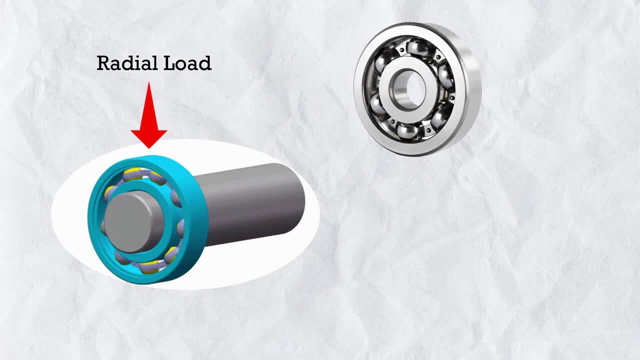 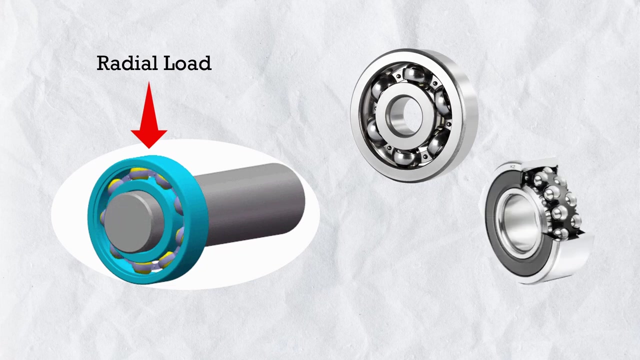 application, like in the same radial motion application, we can use a simple deep group ball bearing or we can also use a angular contact bearing, or we can also use the roller bearings. also there is single group ball bearing and also double group ball bearing. also in angular contact bearing we can use the 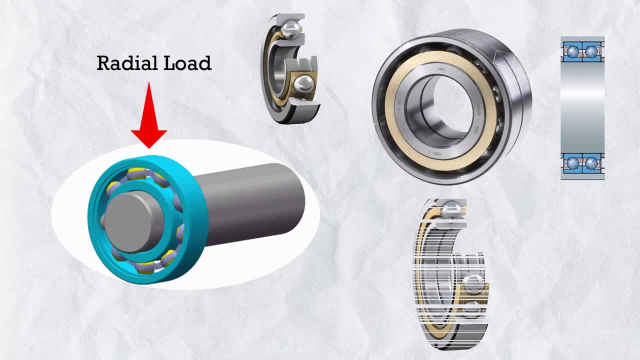 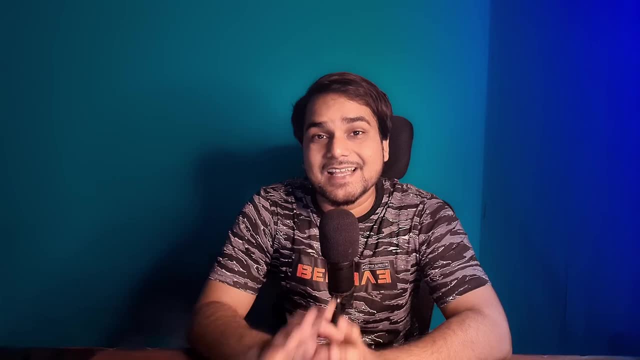 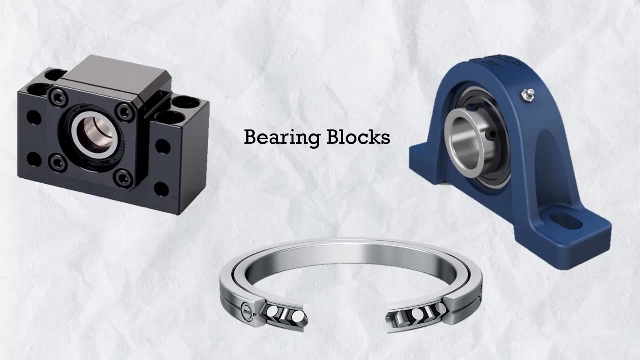 pairs of angular contact bearing or we can also use the four contact angular contact bearing. so we will also try to understand that, how to compare the bearings and select the best suitable bearing. and And later in this series we will also master the different type of bearing blocks. 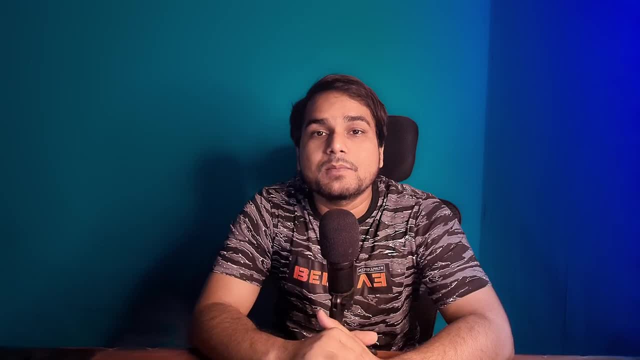 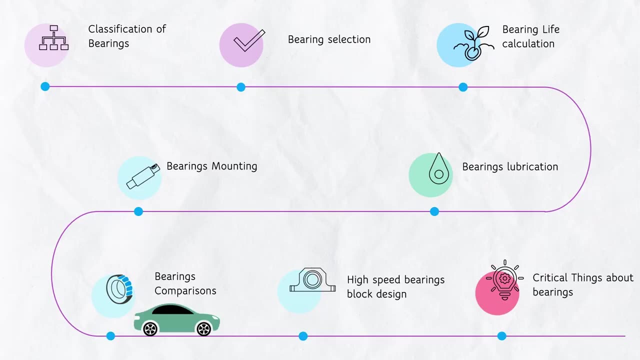 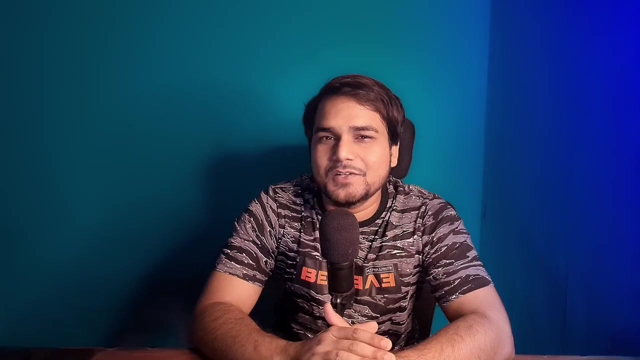 But the standard commercial bearing blocks are usually not available for high speed application Speeds like more than 12000 rpm. So later in this series we will also design a high speed bearing blocks- Speed for 20000 rpm. And to make this difficult we will design an angular contact bearing block. 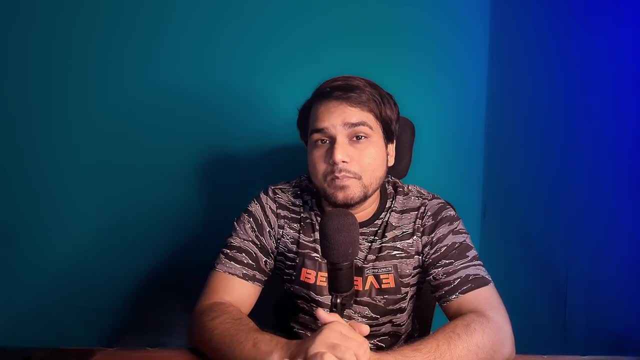 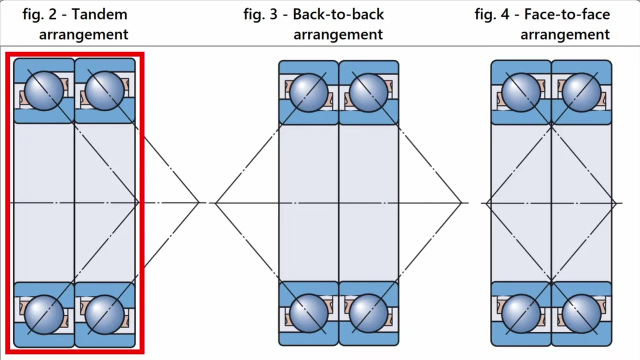 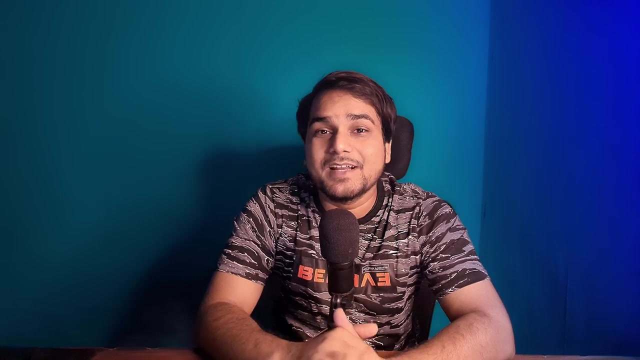 Where we will deeply understand the angular contact bearings and their arrangement, Like back to back arrangement, face to face arrangement or tandem arrangement, And how to decide that which bearing arrangement is better for which application. And then we will comes to know the very critical things. 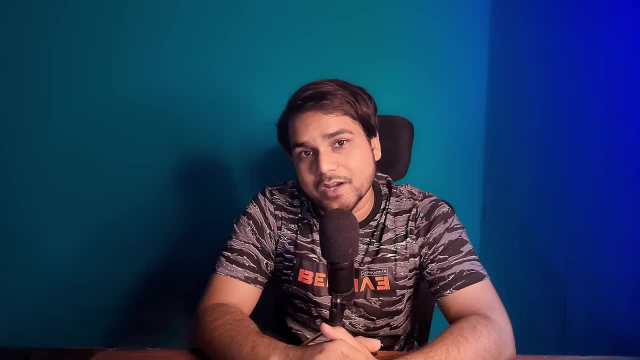 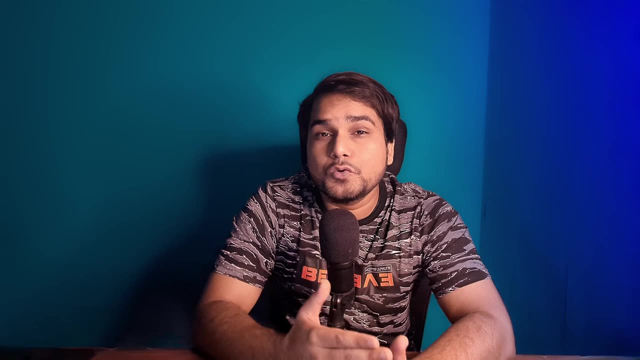 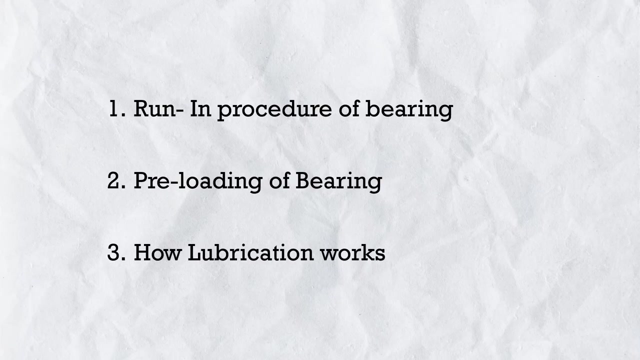 Like why the bearing run in procedure is important and how to do it. Second, the critical role of doing preloading of the bearing And how to do it in the design. And third, the importance of bearing lubrication. That's how the lubrication works inside the bearing. 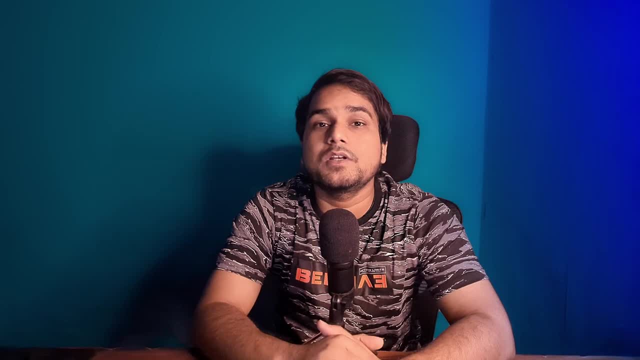 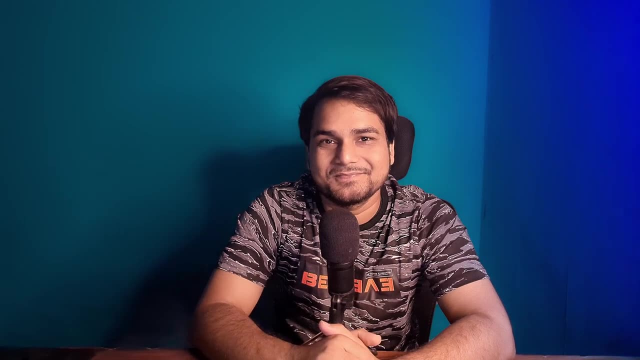 I am telling you, this is so fascinating And these things only few engineers know, Those who have experience in high speed bearing block design- And I am the one. But if you are beginner and wondering, Is that really necessary to know as much about the bearing? 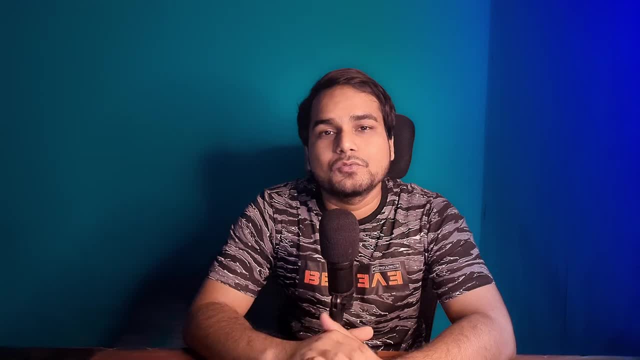 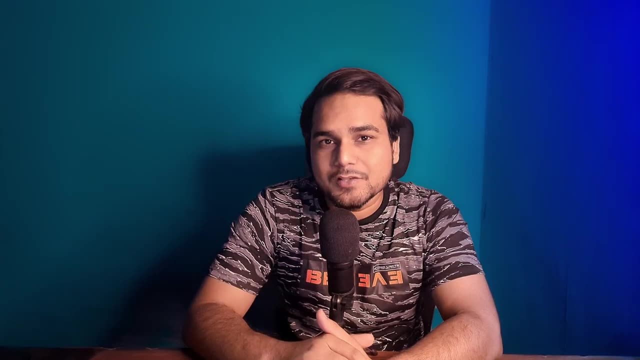 So here is a pro tip For interviews: You just have to know the overviews of all those things Like type of the bearing, nomenclature of the bearing, Or maybe interviewer can ask you the what is the best suitable bearings for a application? 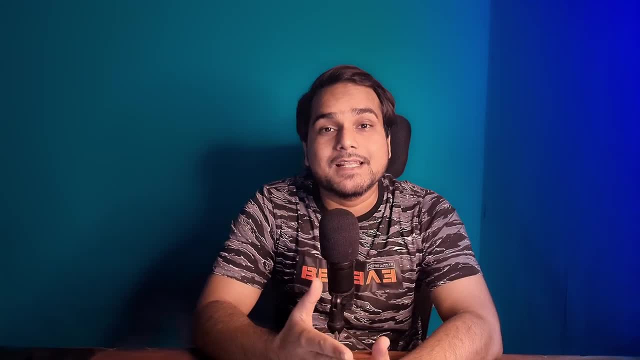 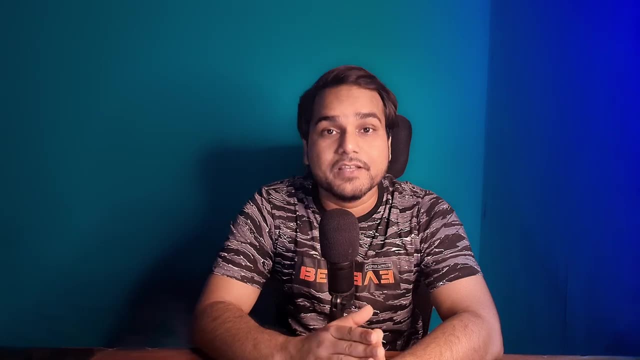 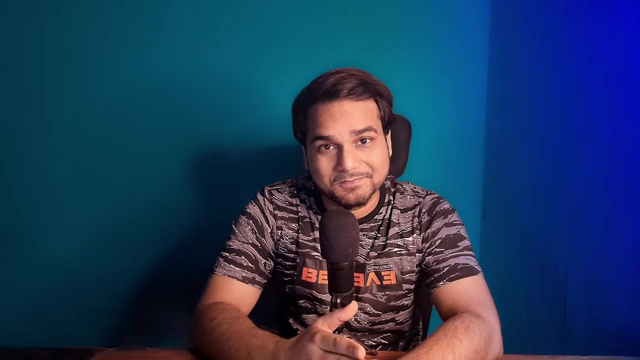 And you will pass the interview anyway. But when it comes to design something critical As a individual designers, it really takes the in depth understanding of everything And we realize the importance of these things. when we design something critical And it fails, I don't know when you failed or never failed in design something. 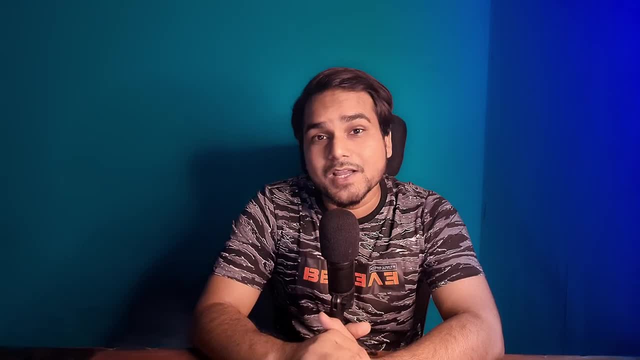 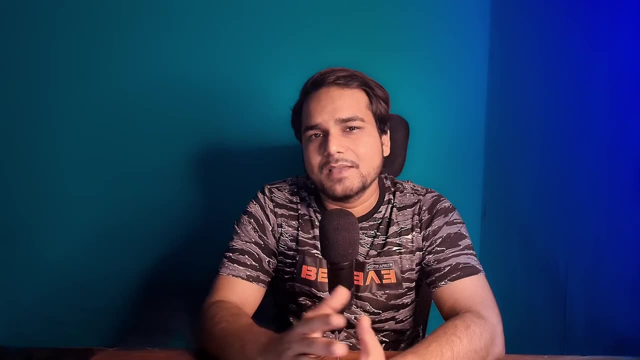 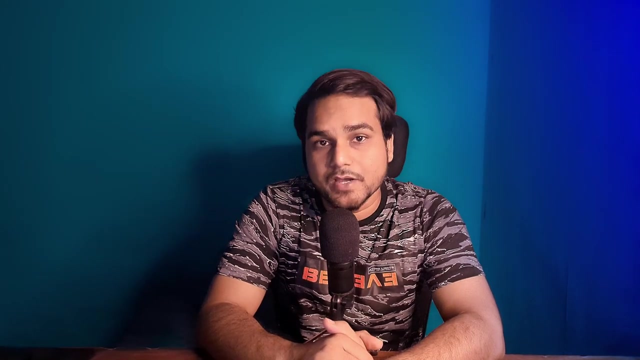 But here is a thing: When our design fails, No one will hesitate to give you the suggestions As per their own experience and understanding, And sometimes even without the complete understanding of your design And in pressure situations. we heard from everyone And we makes the wrong decisions.